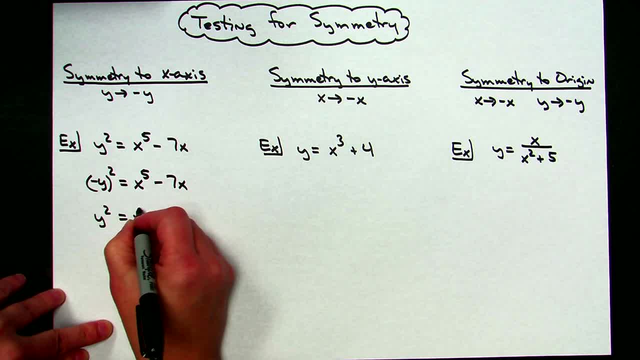 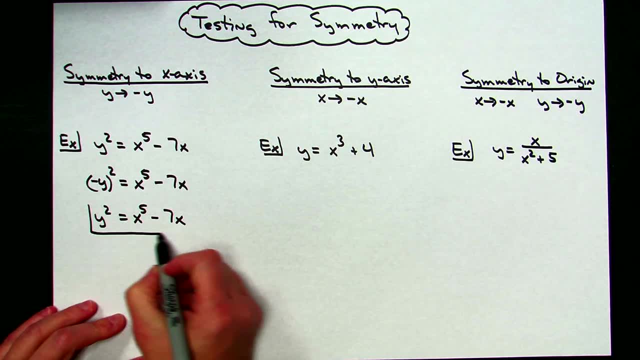 Alright, again, nothing is changing there on the right hand side, so I have an x to the 5th minus a 7x right there. Alright, now once you have simplified. alright, you've plugged that in and you've simplified down to there. 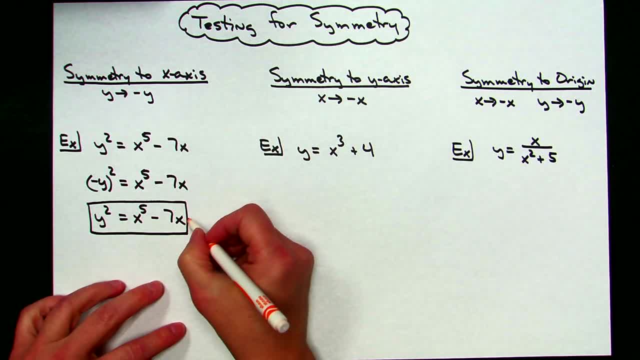 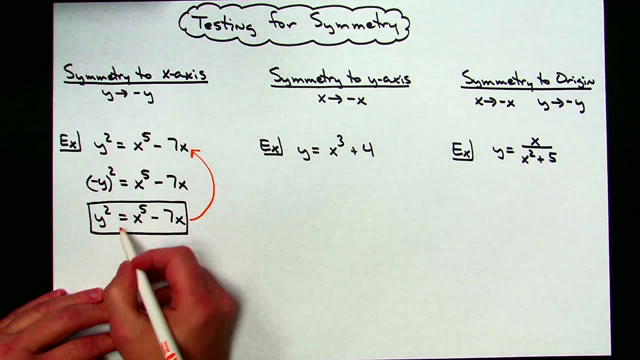 and what you're going to ask yourself is: does this, what you simplified, match the original equation? alright, And in this case, y squared equals x to the 5th minus 7x. It does match, okay, Does it match? 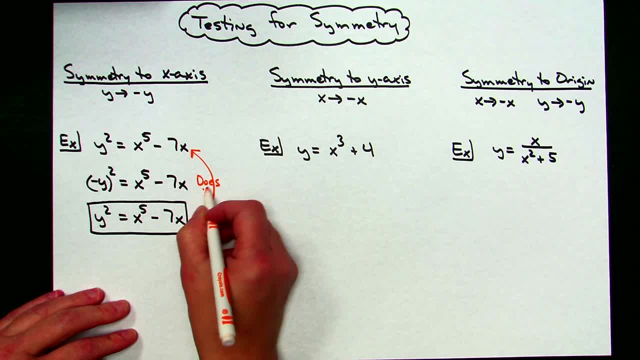 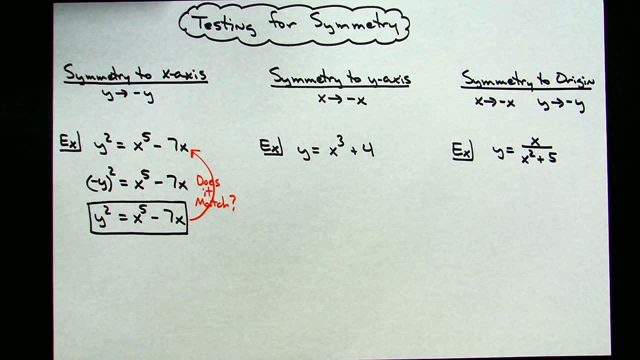 That's the question you're asking yourself. Does it match? Alright? in this instance, yes, it does so. therefore, this equation is: this function is symmetrical to the x-axis, So you could write a little concluding sentence here. Therefore: yes, 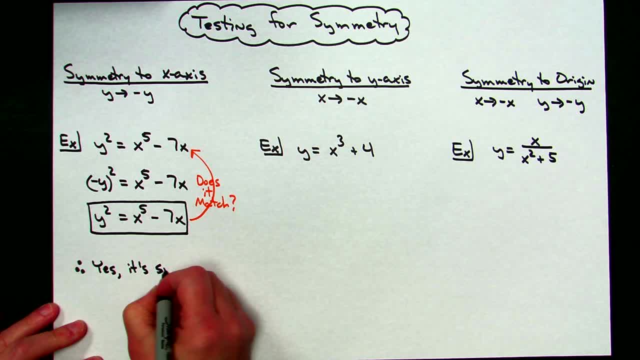 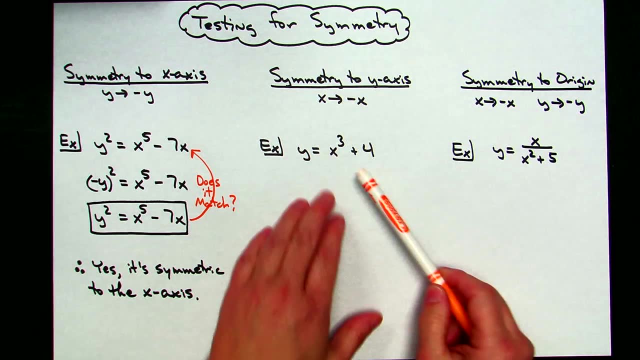 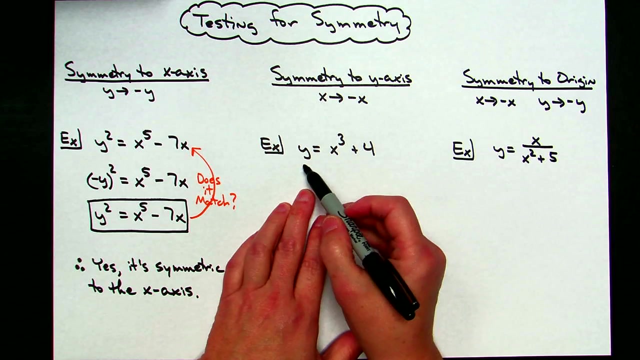 It's symmetric to the x-axis. Alright, now let's suppose I'm running it on a different equation here, just so you can see some different examples of the plugging and the simplifying. Alright, let's suppose I've got this cubic equation: y equals x to the 3rd plus 4,. 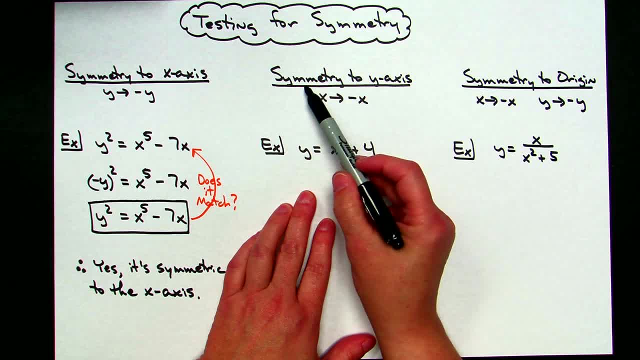 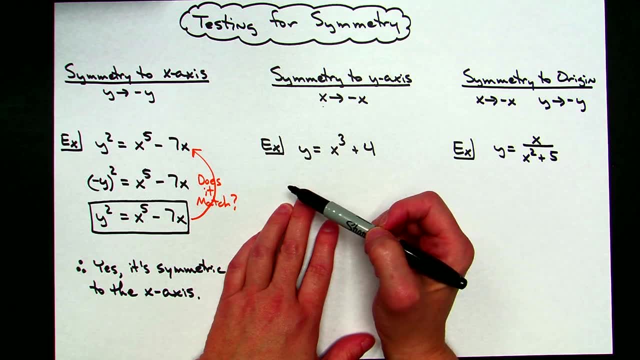 and I want to know if it is symmetrical to the y-axis. Alright, if I want to know if it's symmetrical to the y-axis, I'm going to take every one of my x's and replace them with a negative x and then simplify and then ask myself: 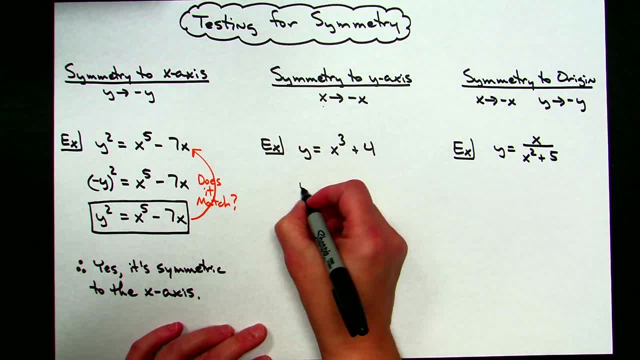 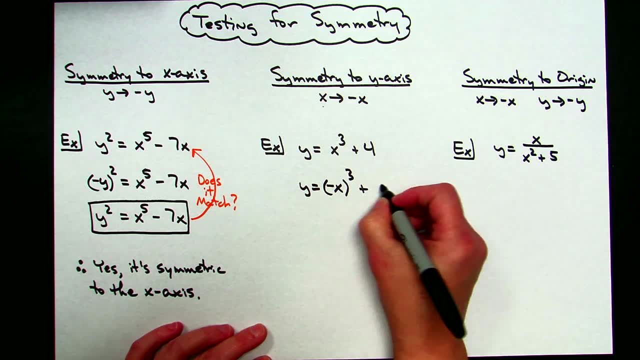 does it match that original function that I started with? Alright, so y equals and I'm going to take that x. I'm going to replace it with a negative x to the 3rd power and then plus 4.. Now I'm going to go through and I'm going to simplify. 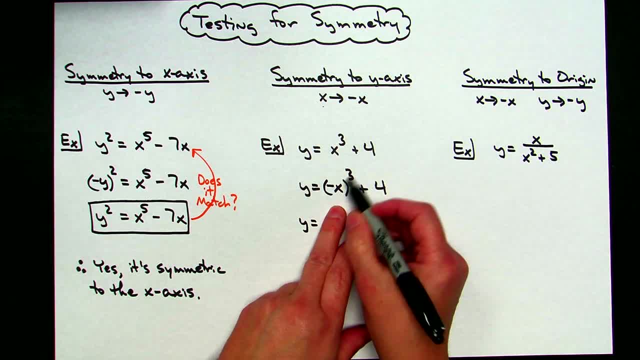 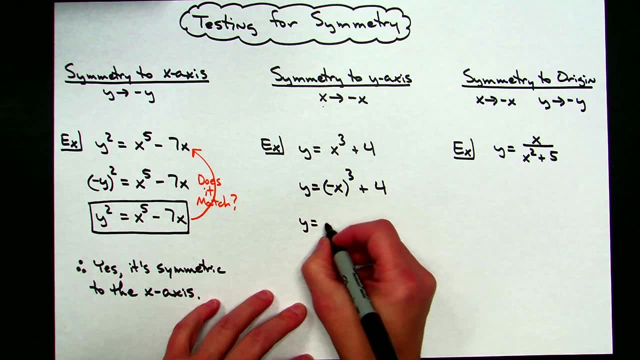 There's nothing to simplify on the left. Alright, now a negative raise to the 3rd power. alright, Anything raise to an odd power, any negative number raise to an odd power, here to the 3rd power, to an odd power, is going to be negative. so then this is going to simplify to a negative x to the. 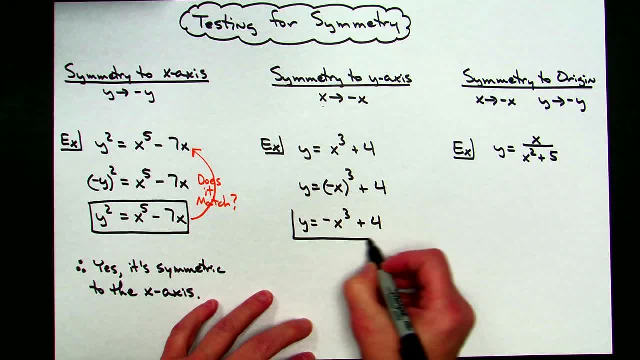 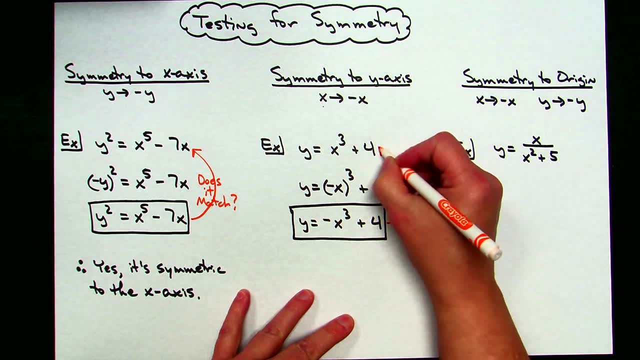 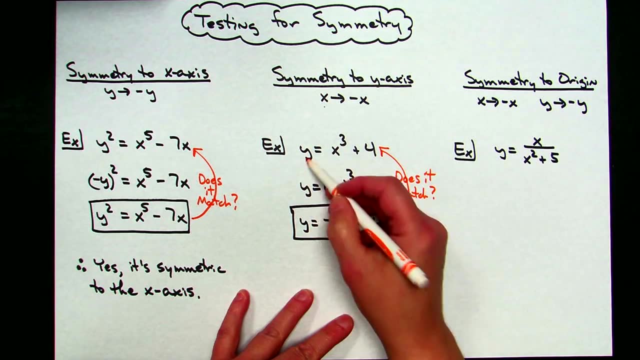 third: all right. and then the plus four doesn't simplify, all right. so I have a simplified that equation down as far as I can, all right. so now I'm going to ask myself: does what I've just simplified match my original equation? all right, does it match? all right? and as we look at this, then we can see: 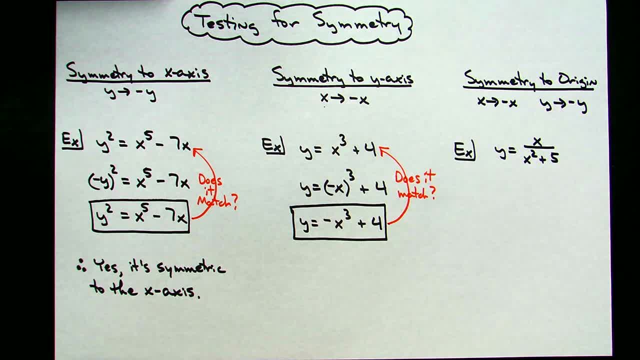 the y is matched, the fours will match, but that x to the third does not. okay, it's positive in the positive coefficient there in the original one, and then what I've simplified here has a negative. all right, so I can conclude that this qubit equation is not symmetrical to the y-axis. 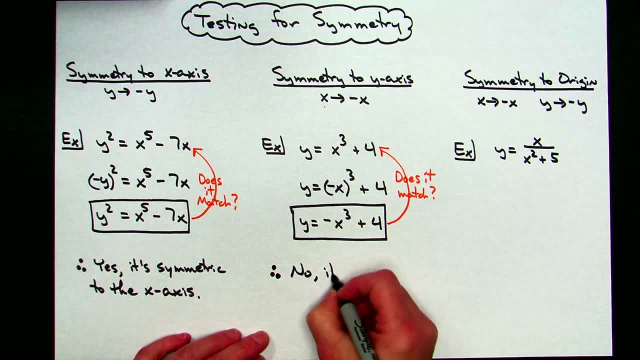 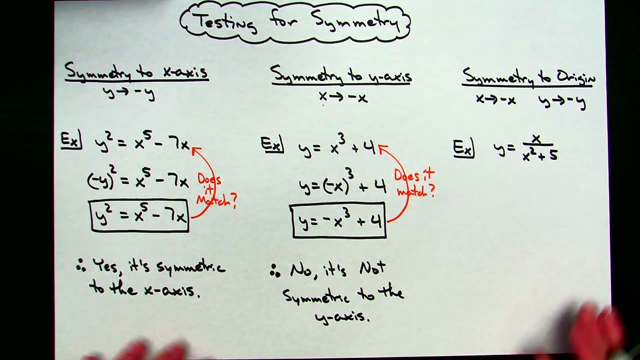 therefore, no, it's not symmetric to the y-axis. and if you happen to have your family of curves memorized and you happen to know that an x to the third basically looks something like that, then you're going to realize that well, no, it's not symmetric to the y-axis. all right, we can also test for symmetry around the origin, all right, and I 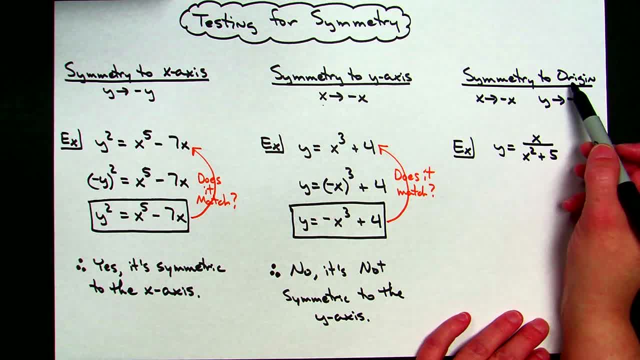 chose a rational function for this example. all right, to test to see if something is symmetrical to the origin. you're going to replace all the x's with a negative x. you're going to replace the y's- all the y's- with a negative y. all right, so my original function here: y equals x over x squared. 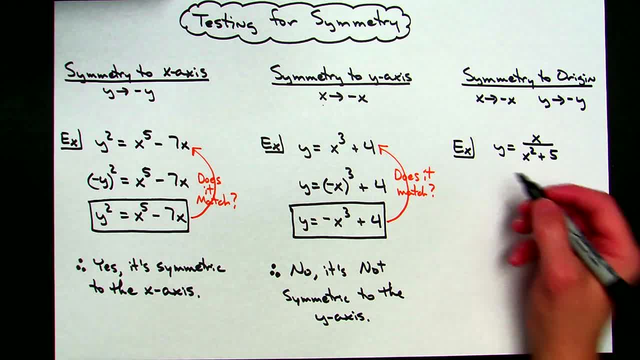 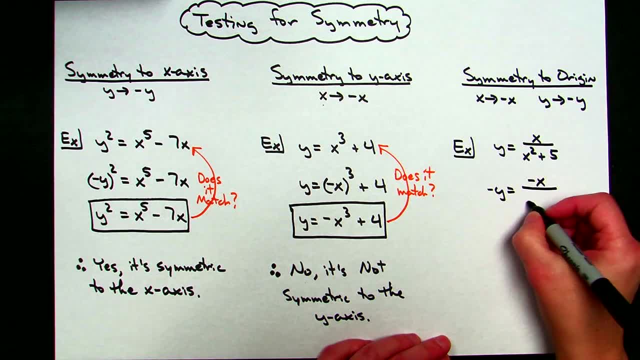 plus five. so I'm going to replace the y here with a negative y. I'm going to replace both of those x's with a negative x. so on top we'll have a negative x down here. on the bottom I'm going to have a negative x squared plus five. all right now. 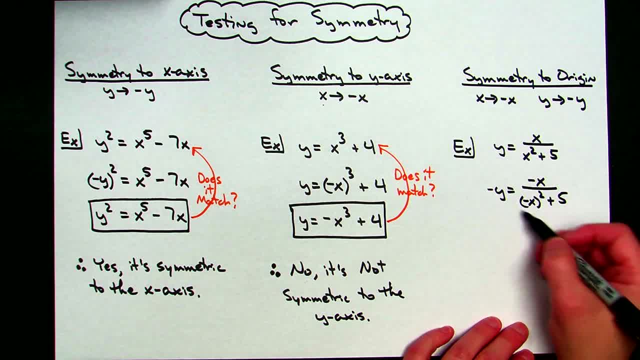 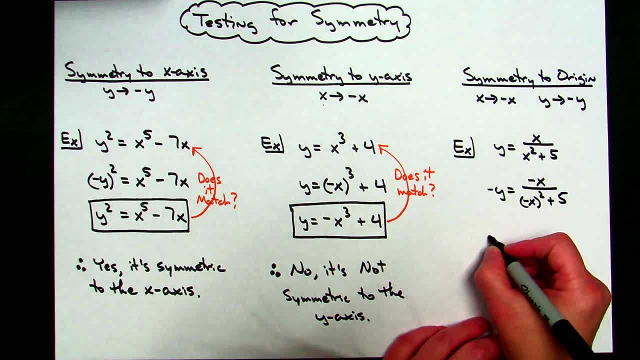 I'm going to go through and I'm going to attempt to simplify all right. first off, and the first thing I want to simplify is that denominator. right there I've got negative x and it's being squared. any negative number squared is going to give me a positive in the bottom, so I'll have 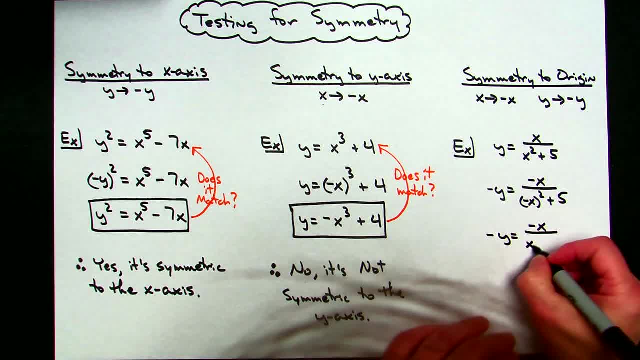 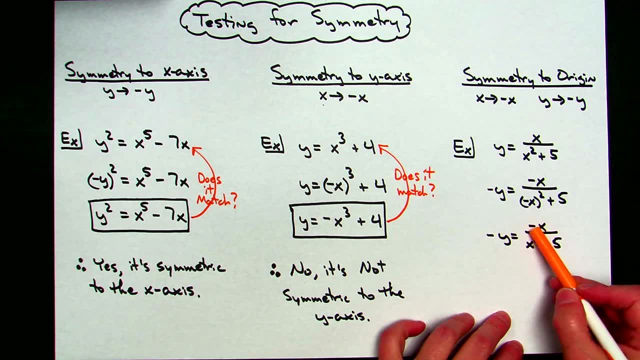 a negative y equals a negative x over x squared Y沒錯 than x superpositive squared plus 5.. All right, now I've got one more simplifying here I can do. I've got a negative on the left-hand side, I've got a negative on the right-hand side, so I can divide both sides of. 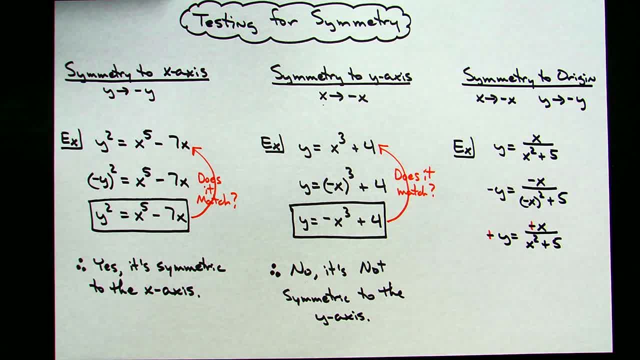 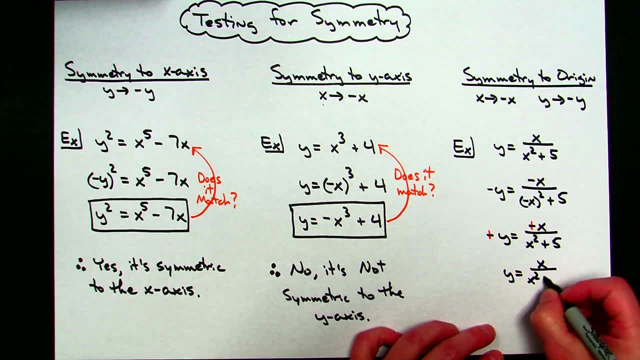 the equation by negative 1, which in essence, is just going to cross those two things out. All right, now I can look at that. I've got a y equals x over x squared plus 5 for my final simplified answer. All right, and again I'm going to ask myself: does my simplified answer?